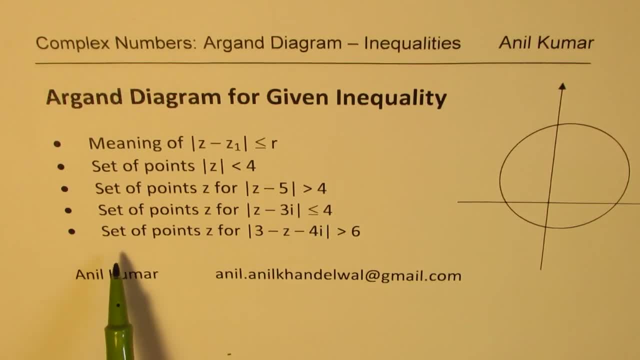 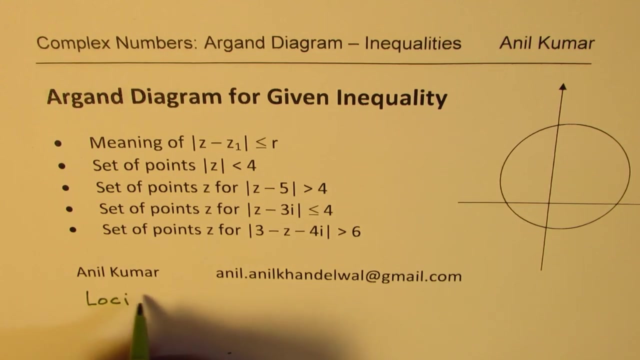 value of Z minus 3i less than equal to 4.. And then set of points of Z for absolute value of 3 minus Z minus 4i greater than 6.. So we say loci as another term, which is set of points. Now, in all these examples we are: 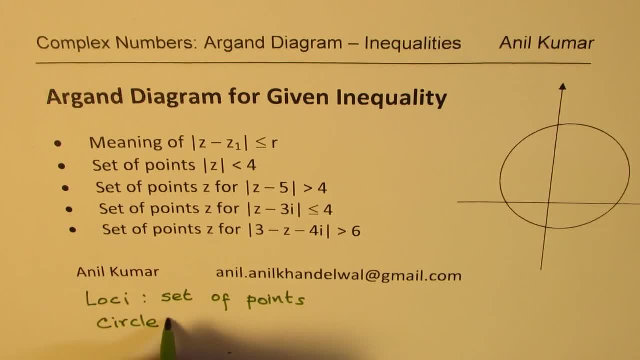 actually sketching circle, right. So that is very important. So what we learned earlier and let me review it here: When I say absolute value of Z minus Z1 is less than equal to R, it means Z1 is our specific vector, right? So let us call Z1, as sometimes we refer this. 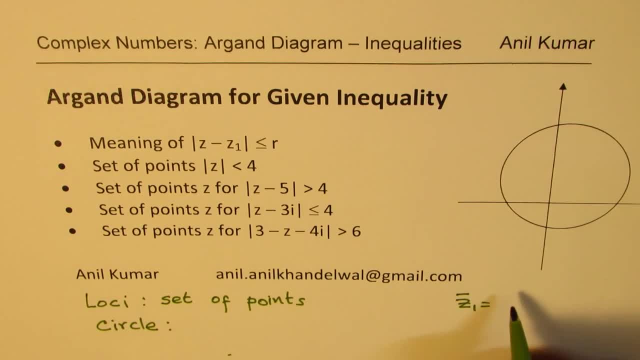 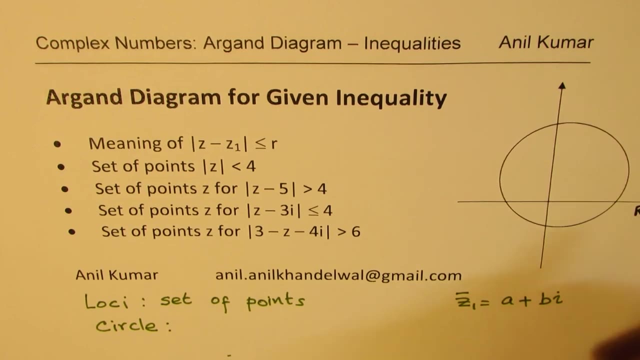 to vectors, but we are not talking only about complex numbers in general, So let it just be a plus bi. okay, So this could be represented on our argon diagram. Horizontal axis will be treated for real numbers, vertical as imaginary. 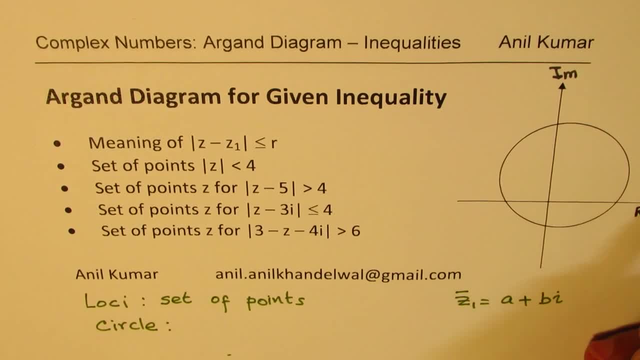 Sometimes we write Iy there and x on this side. So when I say Z is a plus bi, then from the centre the value is a. means go right, real a and then go upright. So we get this point and that becomes the complex number Zi, right? So this represents Zi Z1. I should. 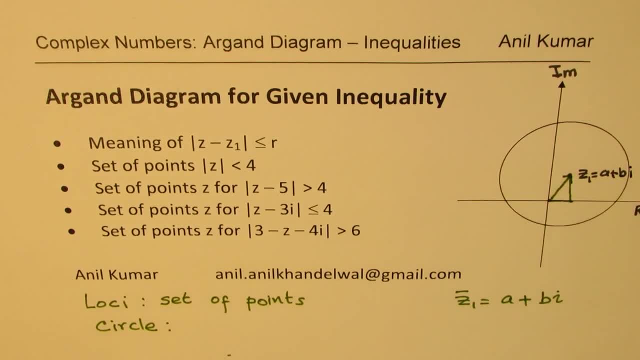 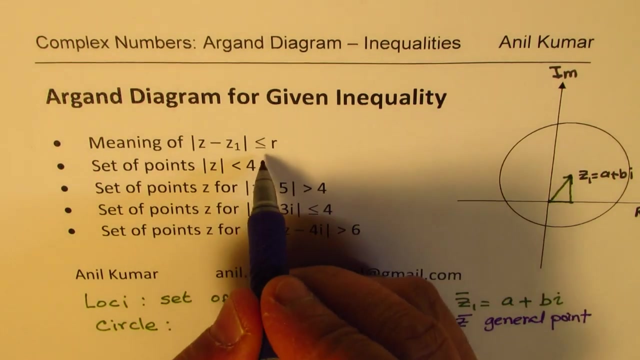 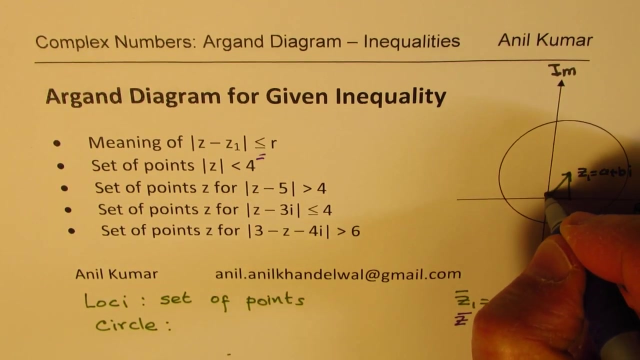 say, equals to a plus bi. Now Z is basically in our space, a general point. So that is a general point. So anywhere, but with the condition- and in this particular case we have a condition and meeting that condition, we will find that it is basically somewhere. 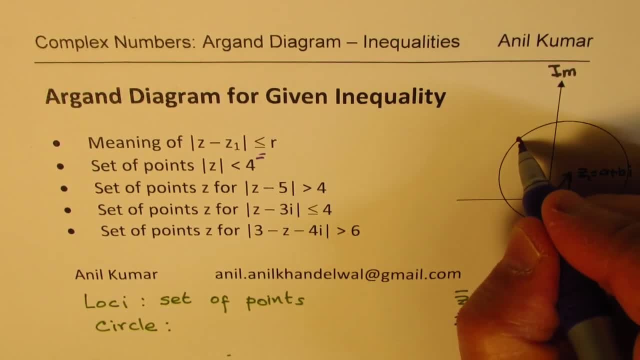 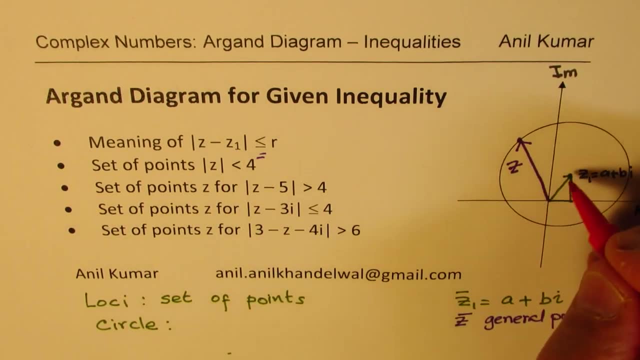 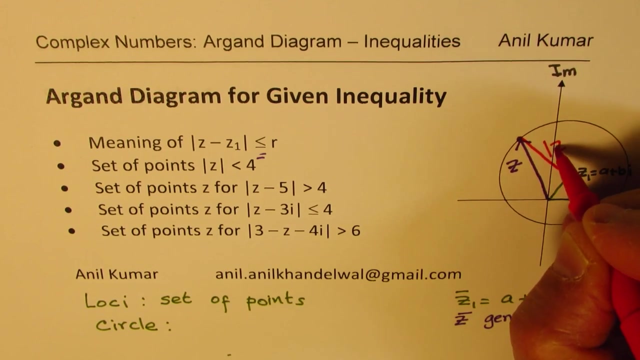 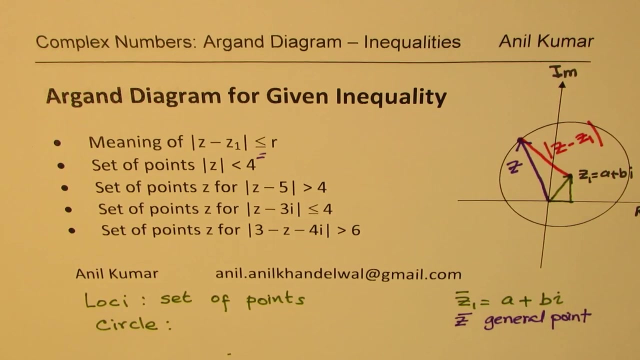 But from this point to within right. So let me first make this as Z, and when we say Z minus Z1, it means this: So this is basically Z minus Z1, correct. Now we have to look into another parameter which we have introduced, and that is the value. 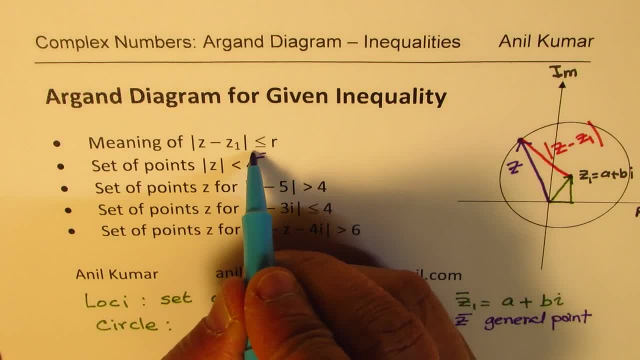 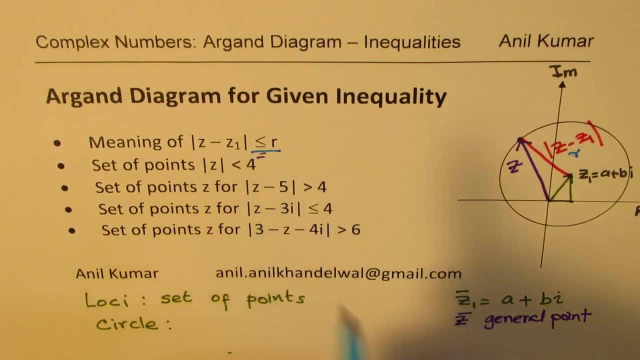 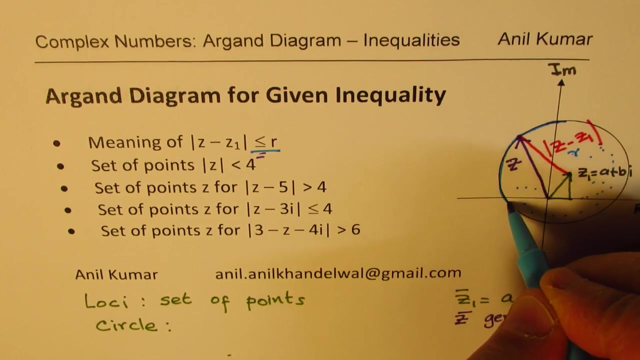 of less than equal to R. Now Z minus Z1 is basically R. So when I say less than equal to R, that means the Z could be anywhere inside the circle, including the points on the circle. So less than equal to means that we are looking for this particular graph. Does it make sense? 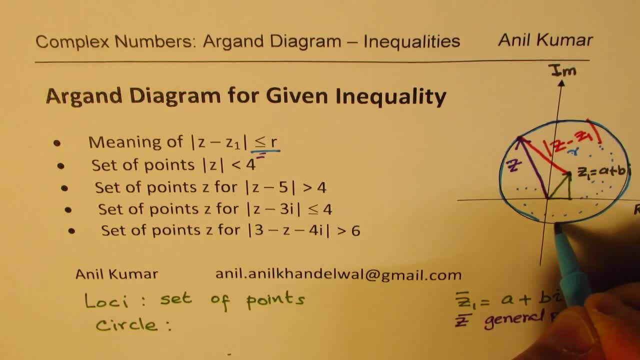 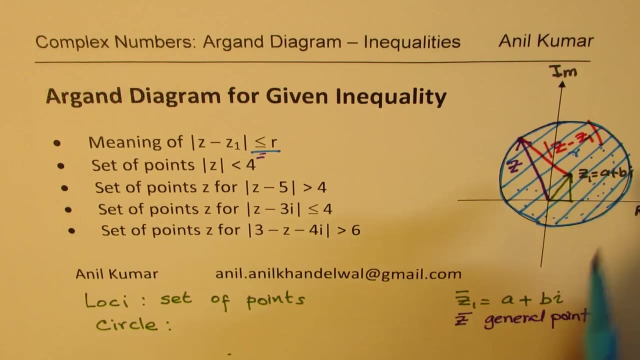 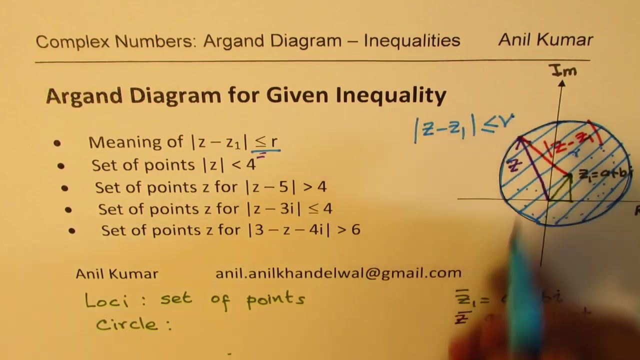 to you, right? So we are looking for this circle And everything inside the circle, Perfect. So when I do that, fill this up. in that case, what have I done here? I have shown Z minus Z1, less than equal to R. Is that clear? So 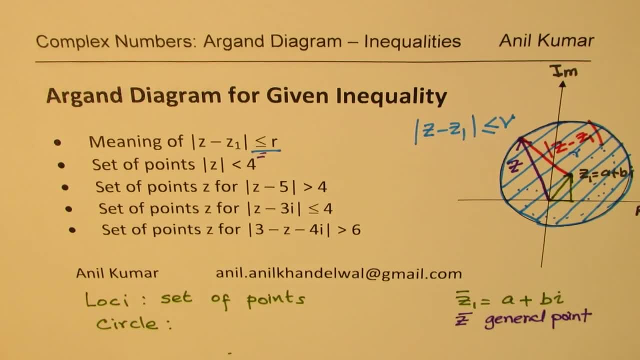 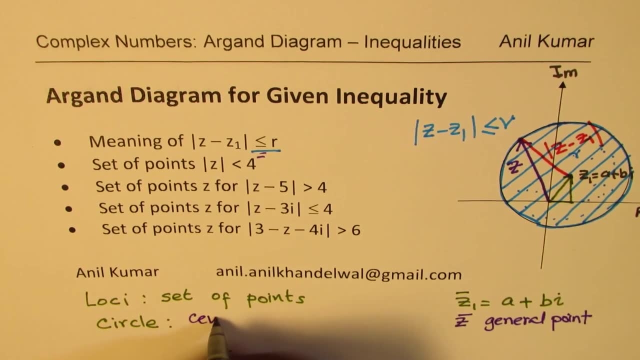 that is how we are going to work and take up all the examples. I hope that is absolutely clear. So this circle which we are talking about will have center, and this center will be provided by the point Z1 and will have a radius, and this radius will be R, the number given on. 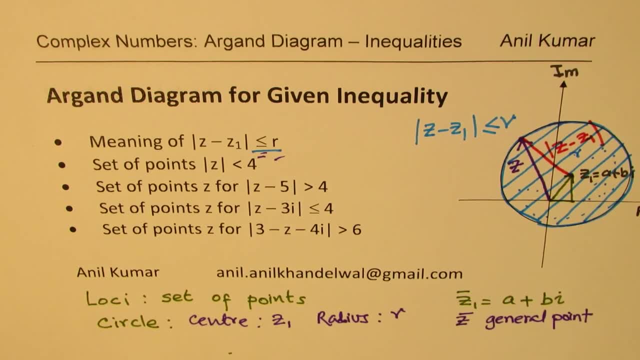 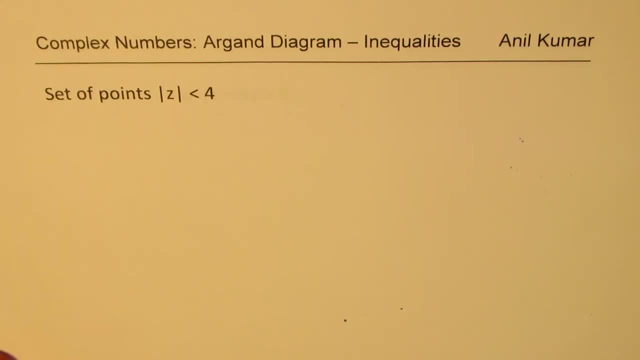 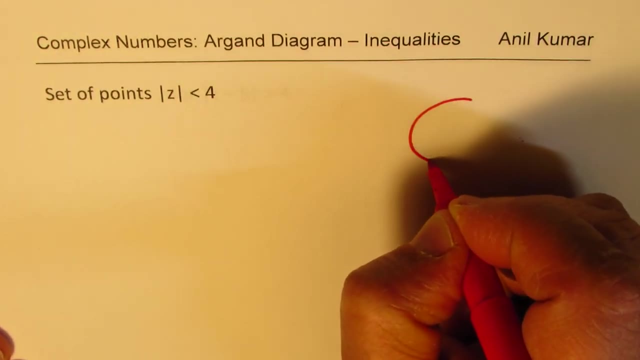 this side Perfect. So let us begin and do these examples one after the other. The very first one here is that we have a point Z1. We have a circle less than 4, right. So that means we can sketch a circle. and where is? 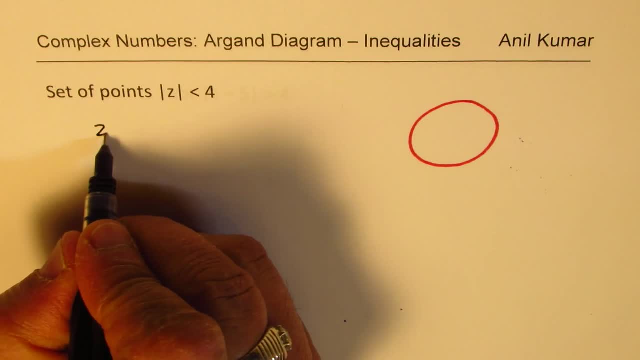 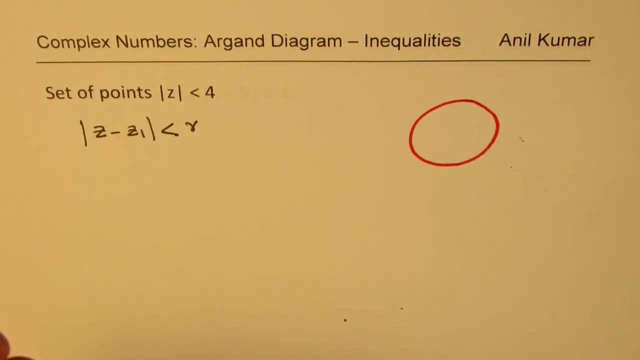 the center for this circle. Well, let us keep in mind the equation Z minus Z1.. In this case, R. we have less than R, correct? So for us the radius is 4 units, right? So this R equals. 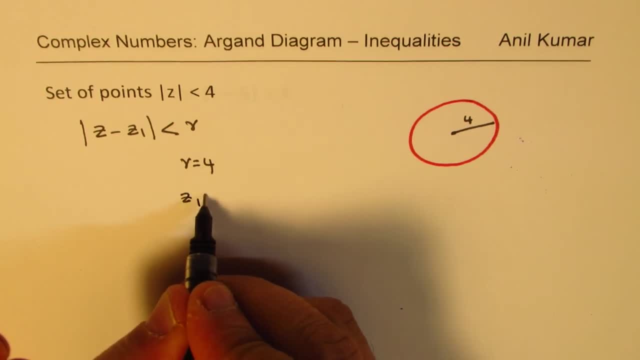 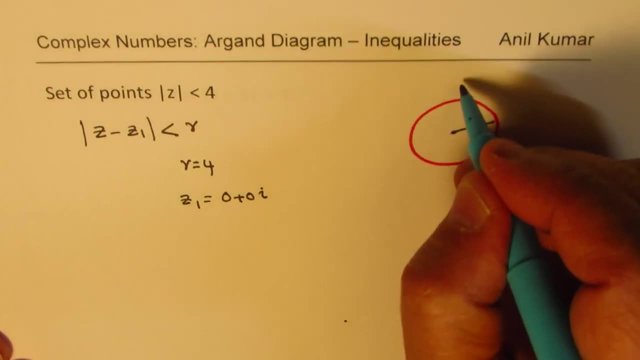 to 4 units. What is the value of Z1?? Well, that is 0 plus 0. So this is the value of 0i. You can say it is the origin right. So basically, this point is origin for you. 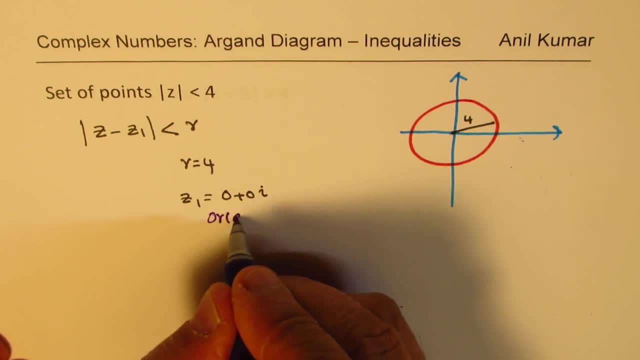 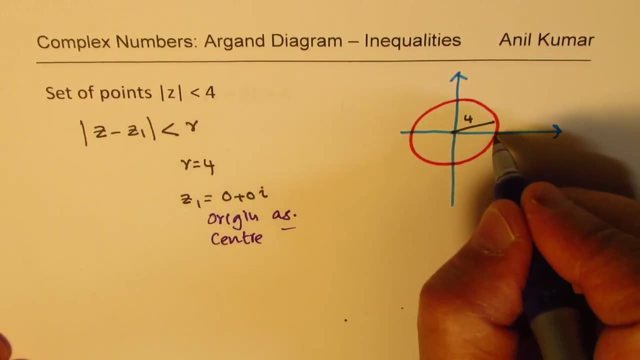 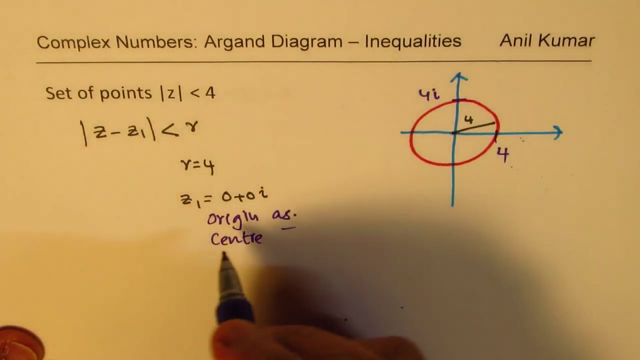 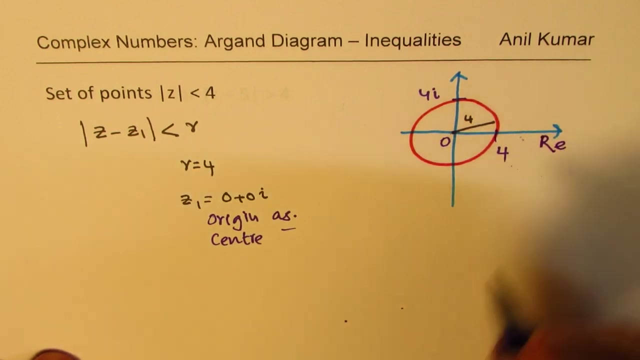 Is that clear? So we have origin as center, clear, And that becomes 4 and this is 4i. Is that clear to you? right? So the radius is 4, right, So that is how you are going to get the sketch right. So this is real. this is imaginary axis. 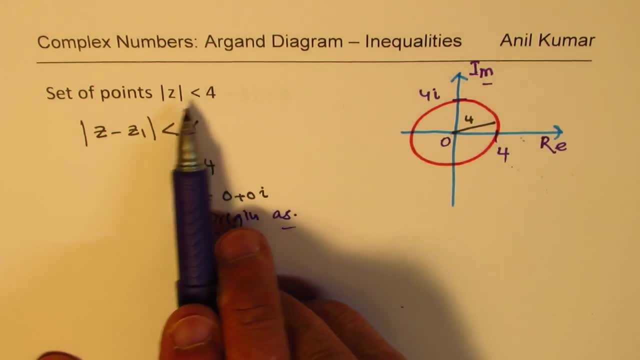 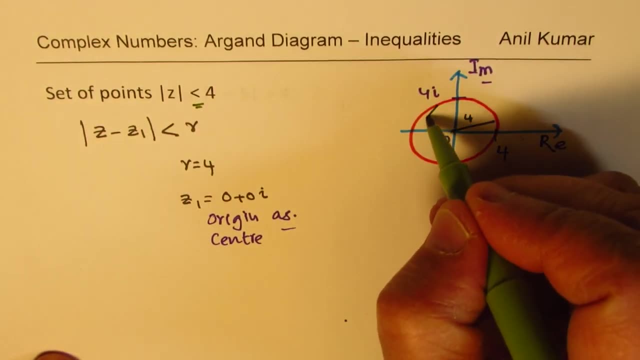 Is that clear to you? So it means everything less than Now. how do you show less than Well when it is less than it means within correct, So it is inside the circle, but circle is not included. So we will have dotted line here. 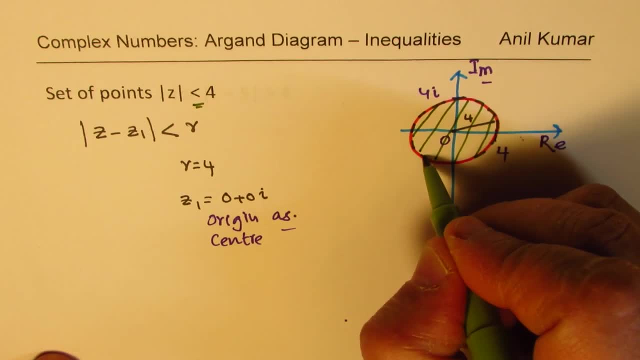 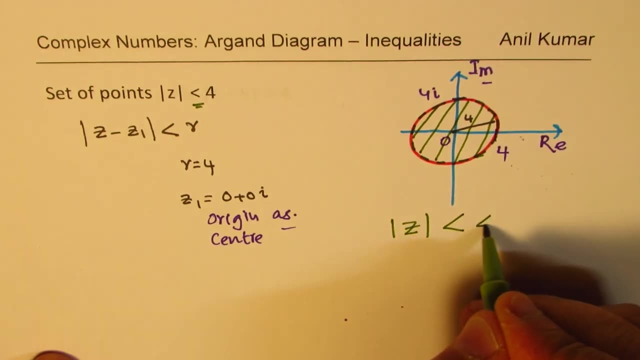 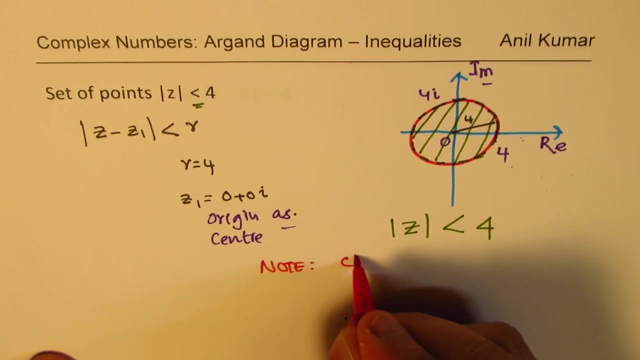 So once I do that, then I am actually showing you the inequality which is Z is less than 4, right? So what you have to note here is that circle circumference not included, So we show it with the dotted line. 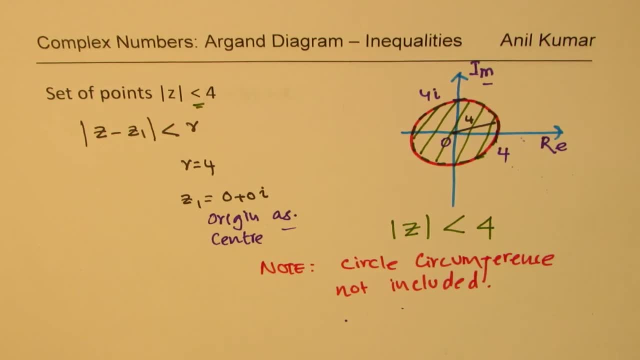 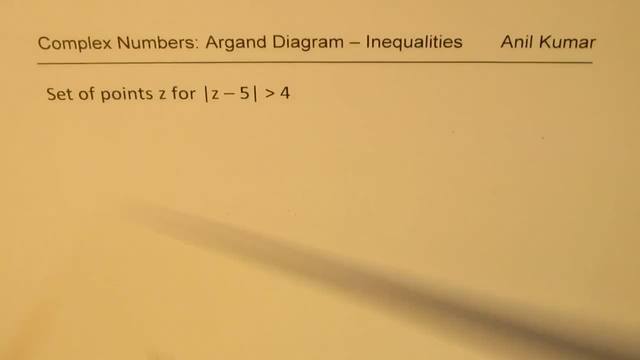 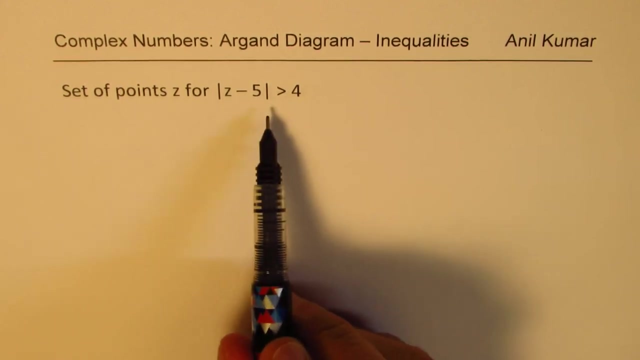 circle. Is that clear to you, right? So inside of the circle, not including the periphery. That's what we are trying to say. Perfect, Let's take the next example now. Now let's try to sketch the set of points z for absolute value of z minus 5 greater than 4.. To understand it, 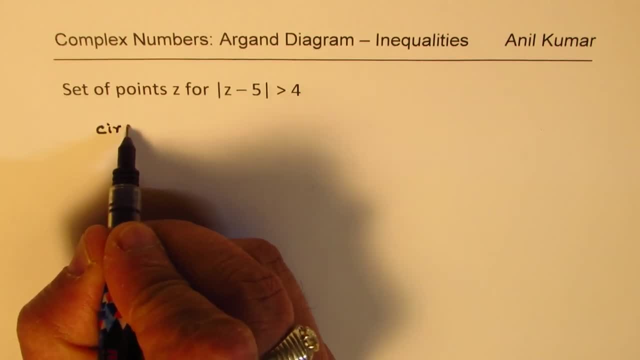 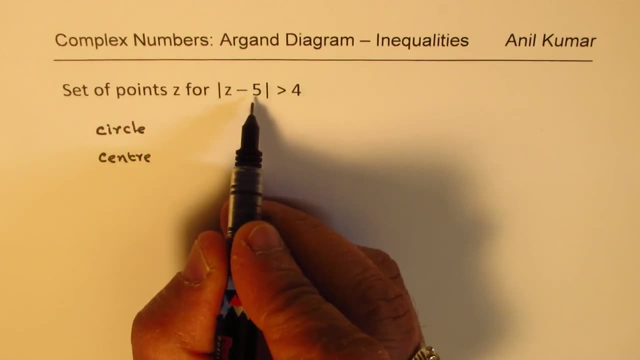 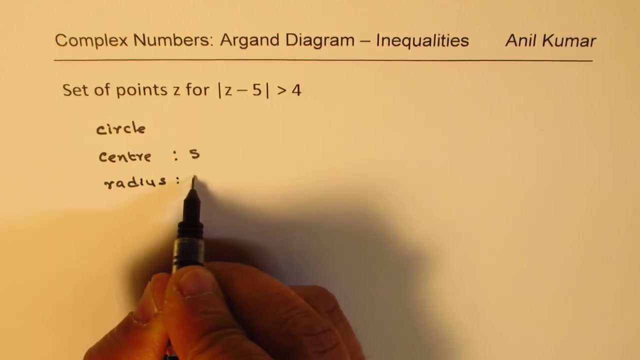 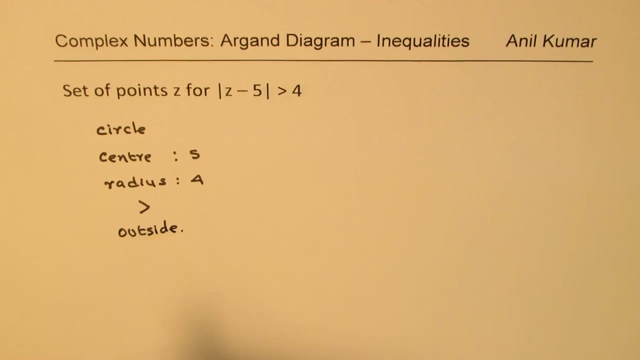 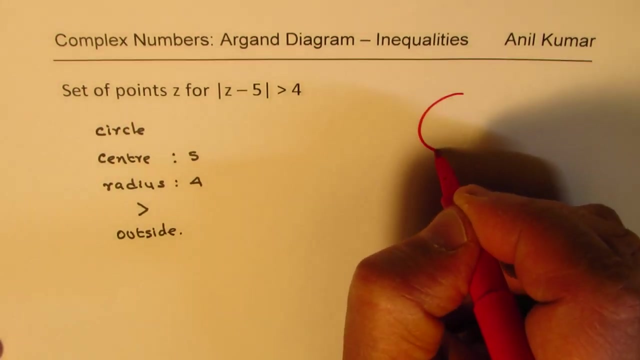 what are we looking for? We are looking for a circle, right, whose center is at 5,, right, So at 5, and whose radius is 4 units, And that greater than means outside. Is that clear, right? So let me just sketch a circle here. So we're looking for a circle. 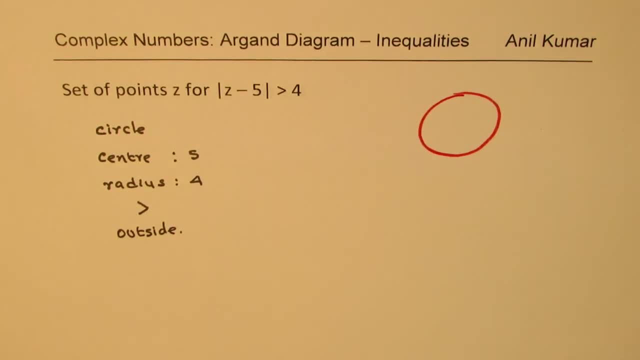 whose radius is 4 units, And that greater than means outside Right, So the radius has to be greater than…. this is the radius right. So when we compare, we are always comparing with z minus z1 greater than r, right? So that is the radius Now. 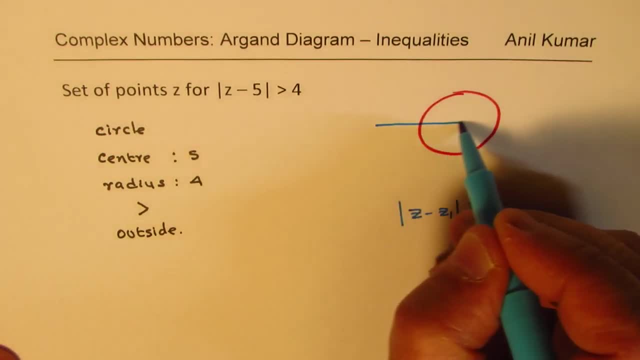 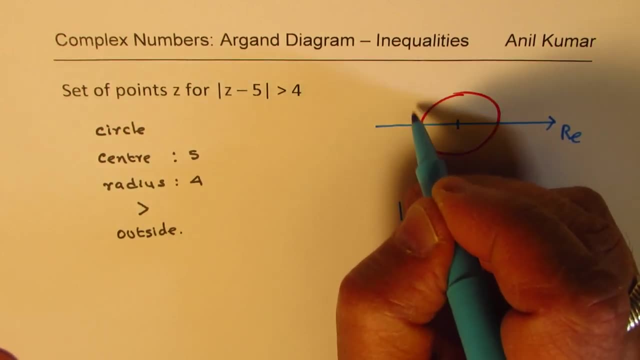 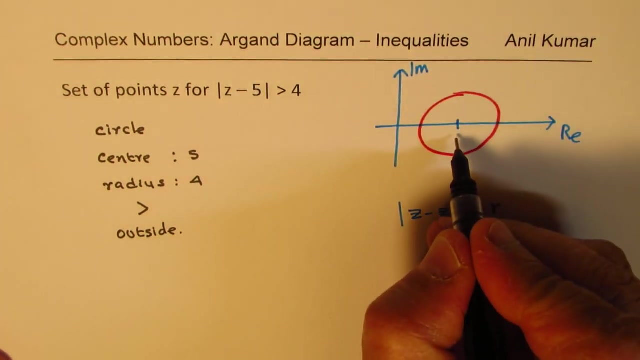 since it is 5 units on the real axis, that becomes a real axis Right. 4 is the radius. so that means somewhere here… will be our imaginary axis. Is that clear to you, right? So this point is at 5. 5 plus 4. 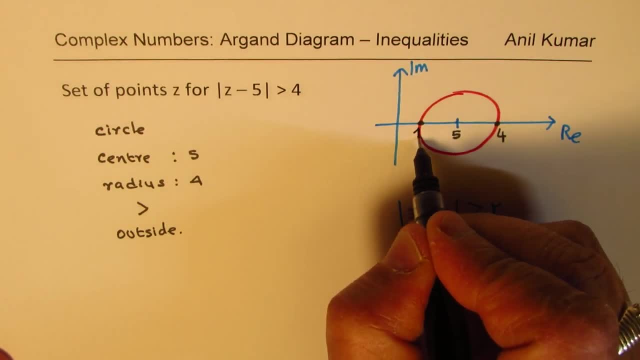 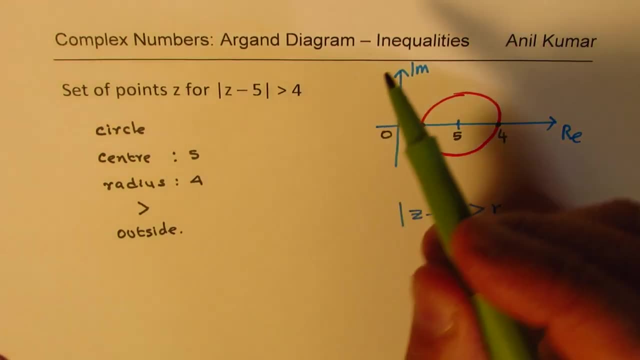 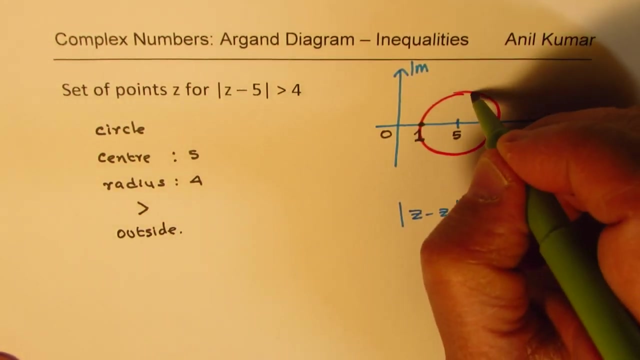 gives you that point and minus 4 gives you this point. Perfect. So that defines a circle. Now, when we say greater than 4, it means what It is outside right. So it is outside this. So 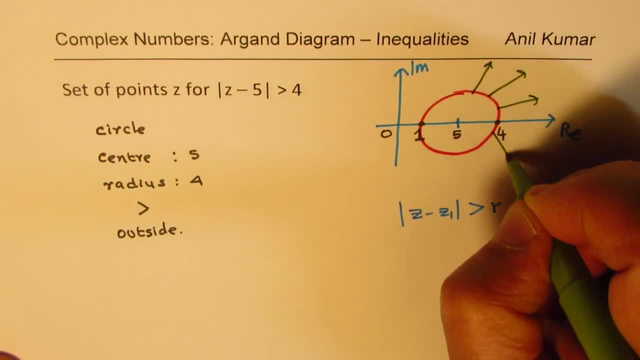 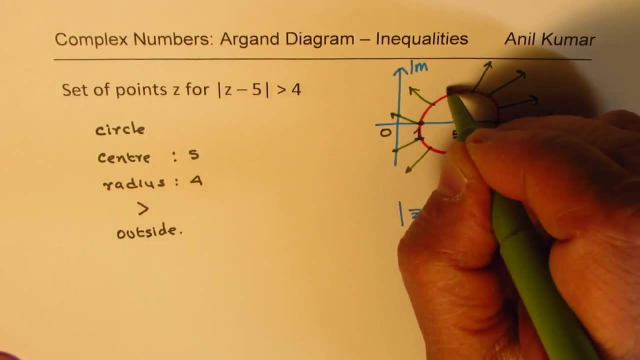 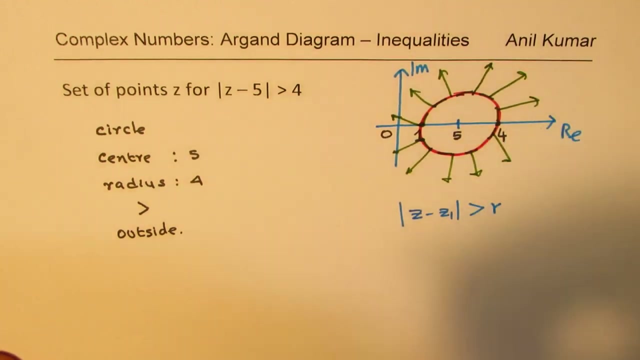 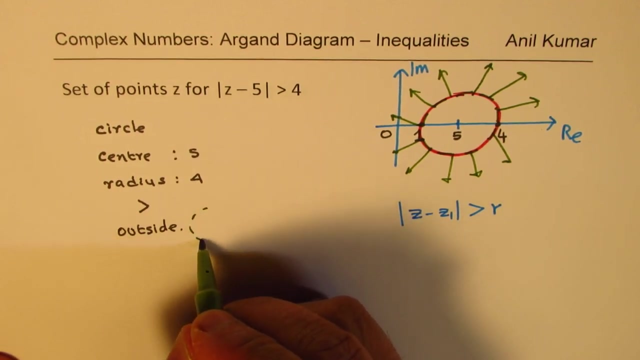 all is outside, where points on the circle are not included. Is that clear to you? So if they are not included, it's a good idea to put this dashed line here. Solid means included, Is that clear? So outside. So outside means circle is dashed. 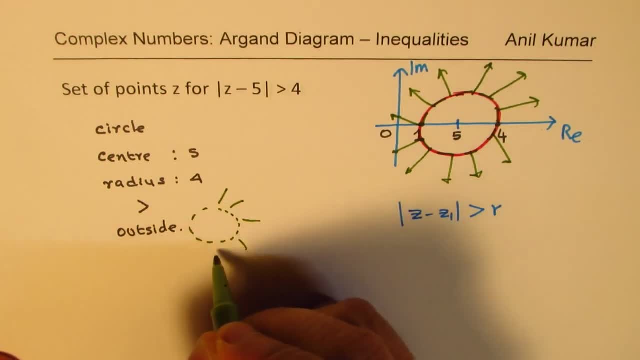 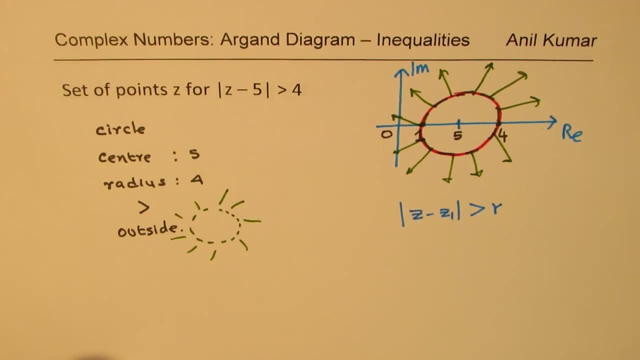 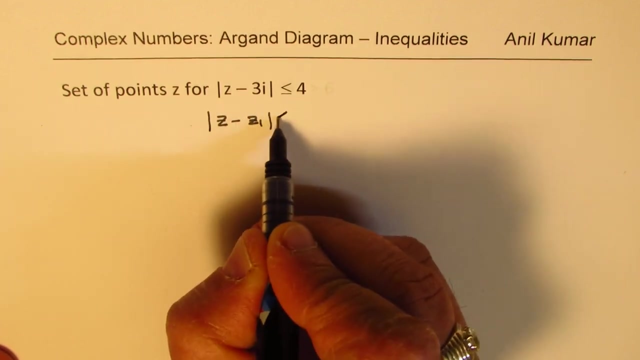 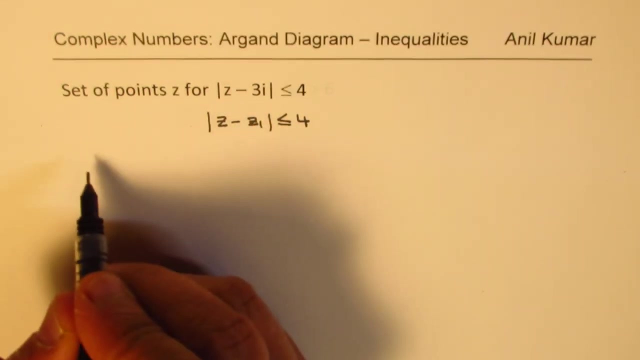 not including, and all this Perfect. So that is how you are going to show the represent the inequality on Ergen diagram Clear. The next one here is z. We have to compare with the standard equation. It's always better to standardize things Now here. in this case, as far as the circle is concerned, the center is where 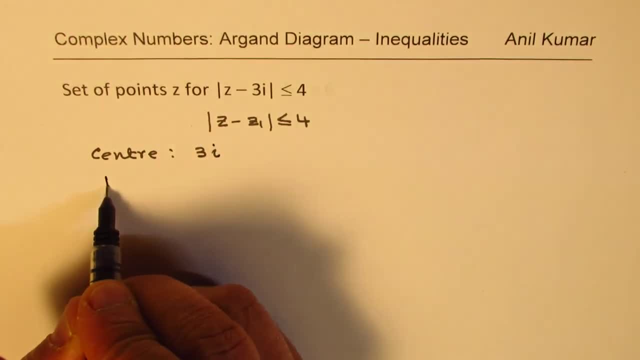 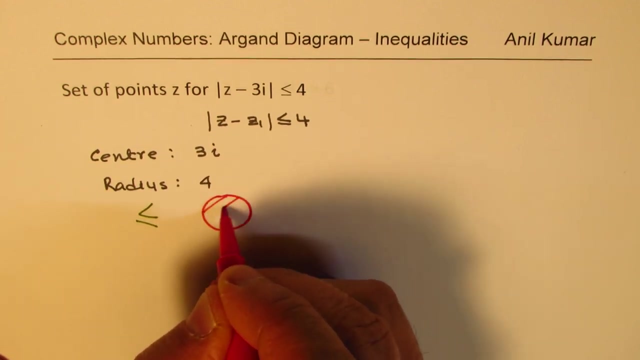 So in this case, the center is at 3i. What is the radius? It's 4.. And what type of inequality we have? The inequality shows that we are working within, where everything is included. Do you see that? So that is what we are looking into. 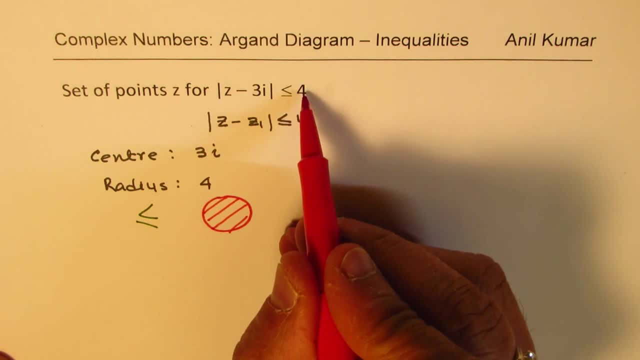 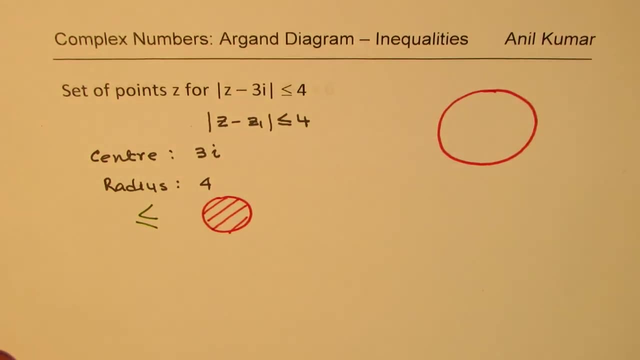 Now let's try to sketch the circle with radius of 4 units and center at 3i. So it is on the imaginary axis that it has a center. so let me just draw this imaginary axis now, since the distance from here is three units, but the radius is for this time. so 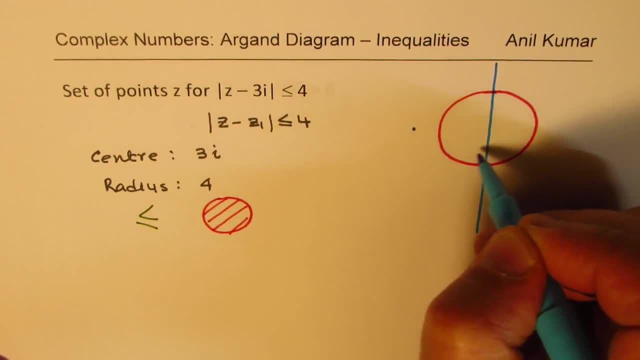 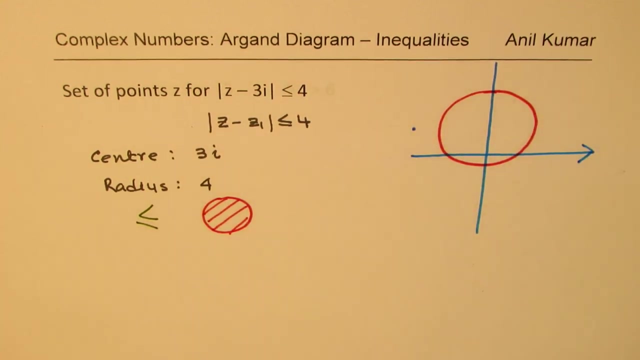 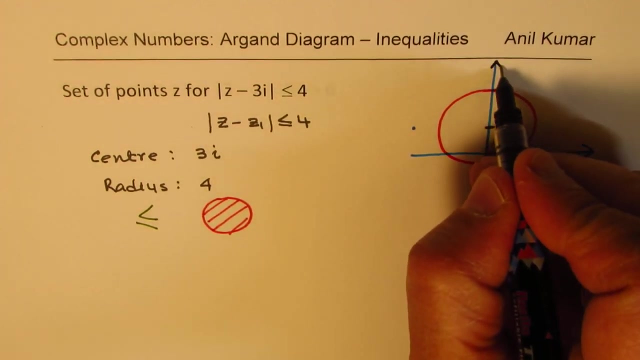 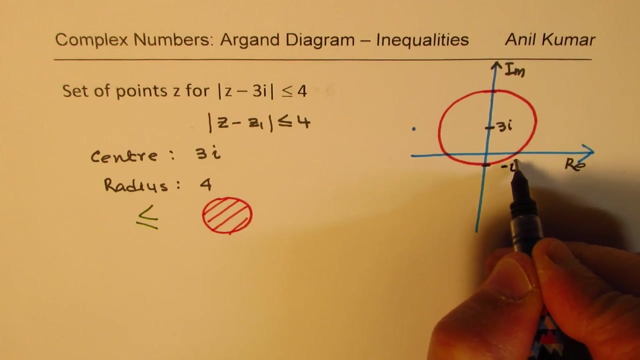 that means a circle could be crossing the x-axis correct, one unit below right. so so what should we have? so that means this: from here, it could be something like this: okay, so from here, the this is 3i for us, right. this is imaginary axis real and that point will be minus. I is that clear. 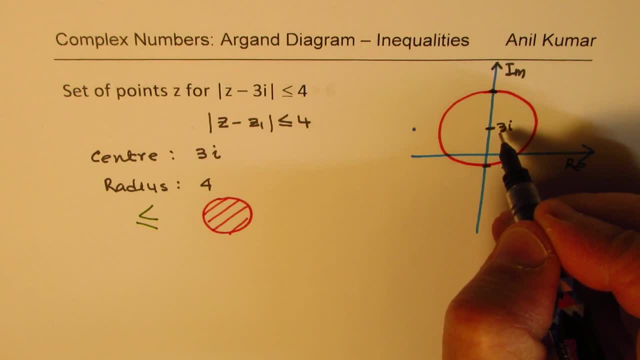 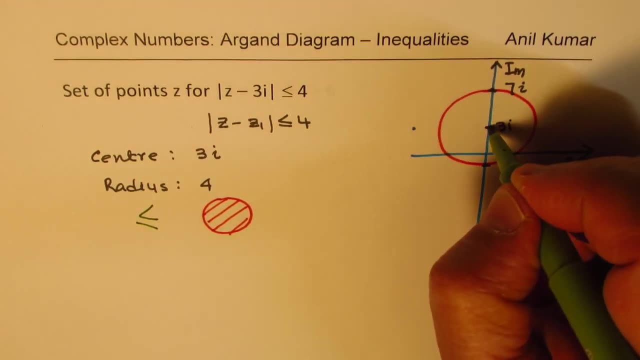 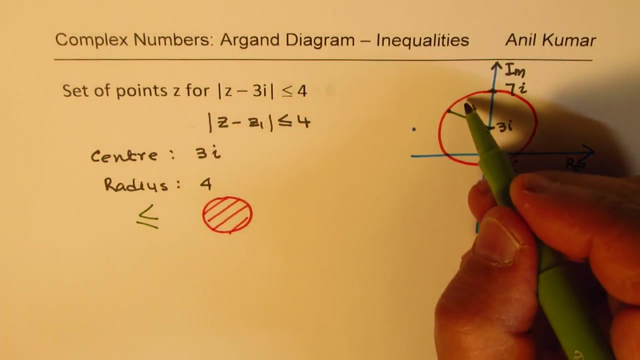 to you, that gives you, and that should be 3 plus 4, which is 7. I got it right. so that is how we ensure that this radius here is for you has to be between 3 and 4 units, and when we say inside, that means everything. 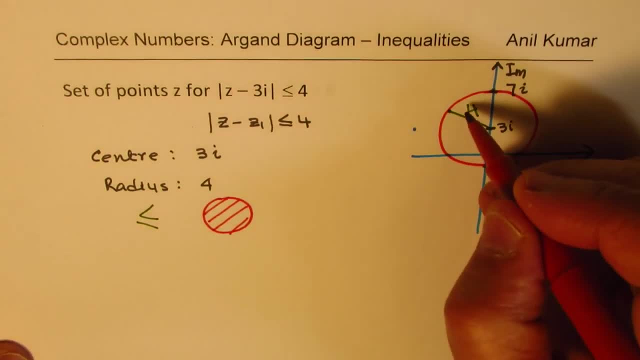 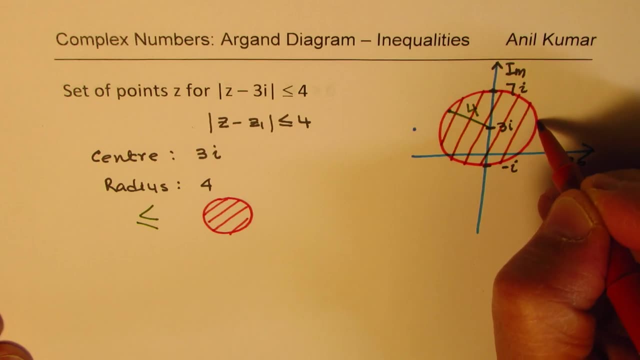 inside, so you have to share it up and including the periphery, right? so it is kind of like this. So I hope the concepts are absolutely clear, right? so this circle is included. is it clear why? because we have this less than equal to, so equal to means. 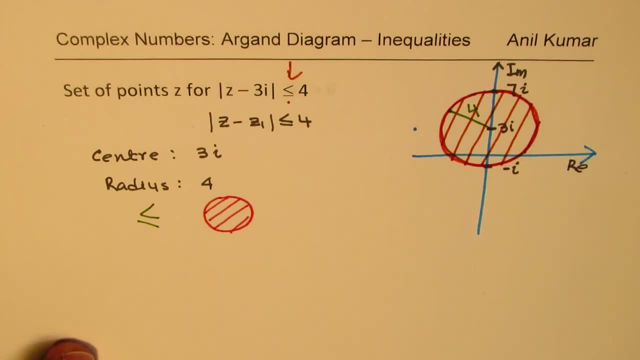 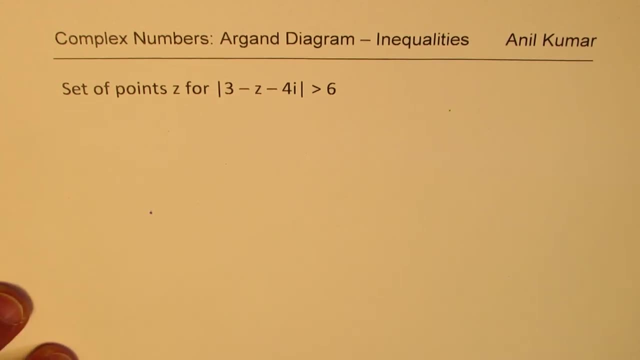 included and if so, мир ut it a. so we did. younger blacks people called it side to side shrimp. they Included perfect. So I think by now you have grand practice on this. Here is your test question. I like you to pause the video right and then sketch this one. so that's your. 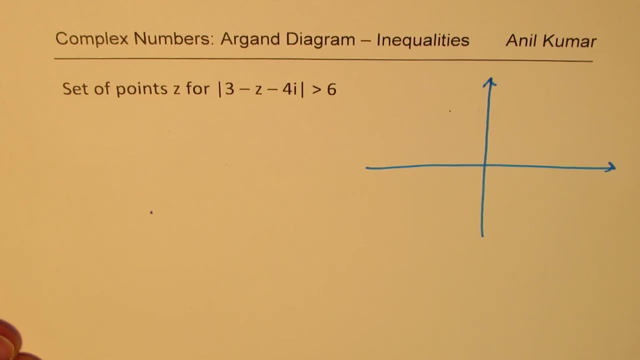 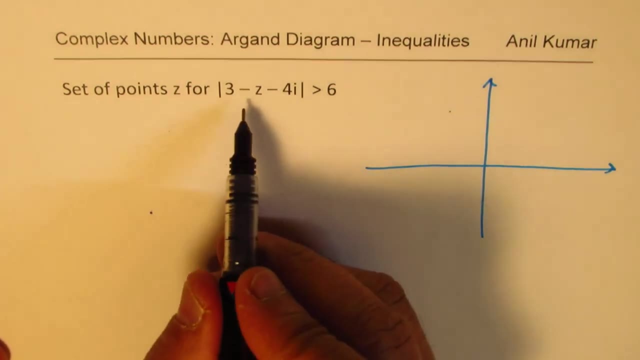 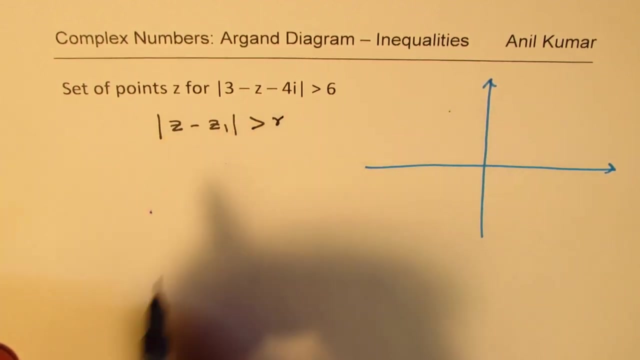 Plane for the complex numbers, you need to draw the argand diagram representing the given inequality. now, in this inequality, First step is to write in this particular form, Then I think the things will be absolutely clear: Z is with a negative sign, So we have to take care of that. so let's rewrite this: we are given 3 minus Z. 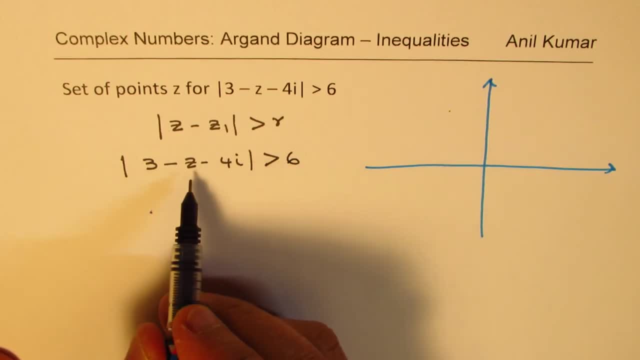 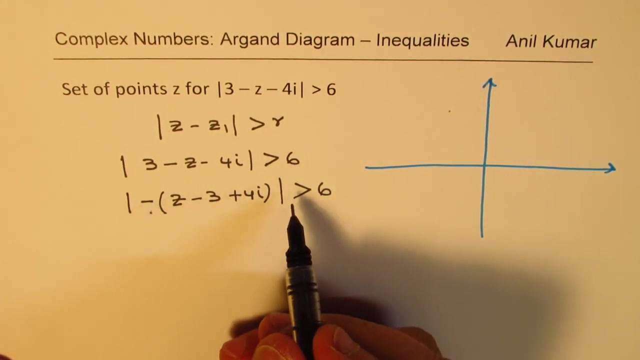 Minus 4i is greater than 6, so we could take the minus common. So we get Z here with positive sign. all of the signs reverses right, so this becomes 4i. Now absolute value of negative 1 is positive, so we could straight away write this as Z minus 3. 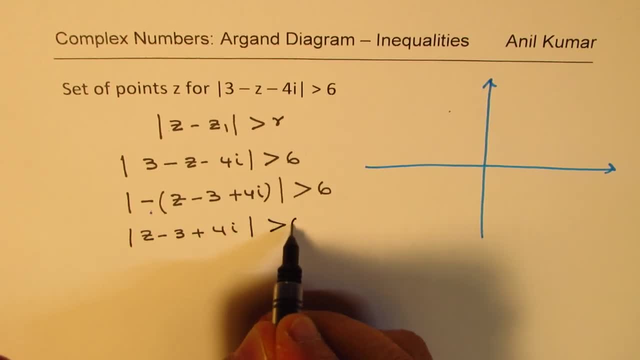 plus 4i correct. Now we need to put this in bracket because it is Z minus Z 1, so it is Z minus 3, and Change the sign 4i. is that clear to you, right? so so lot of steps involved, And that is the type of test question which you might just get. 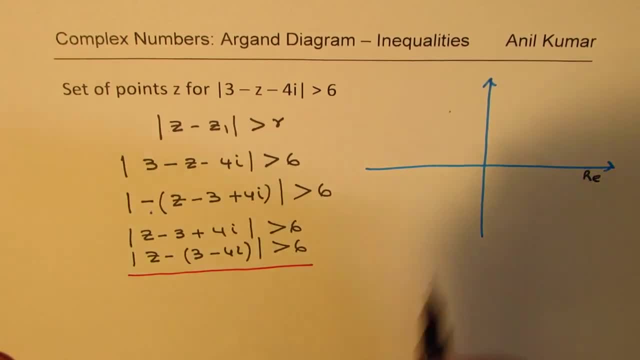 Now I would like you to pause the video and sketch this out. So what is this? at present we have the center Center will be at 3 minus 4i and the radius is 6 units. when I say 3 minus 4i, that means 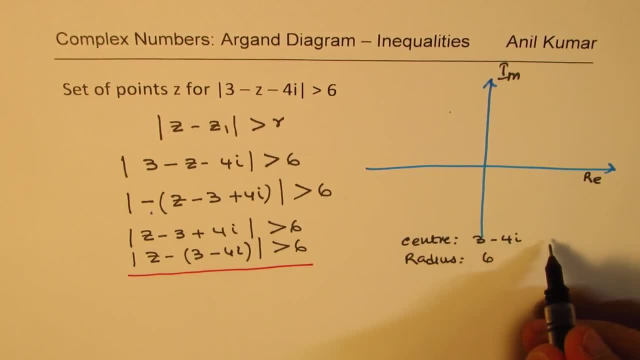 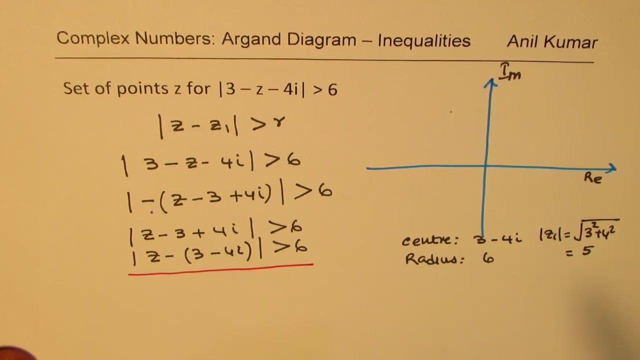 What is the absolute value of Z 1?? Well, that gives you Z 1 absolute value Of 3 square plus 4 square square root, which is 5, correct, 9 plus 16 square root. So 5 is less than 6. Okay Now, 3 minus 4i. so let's get this point: 3 minus 4i. 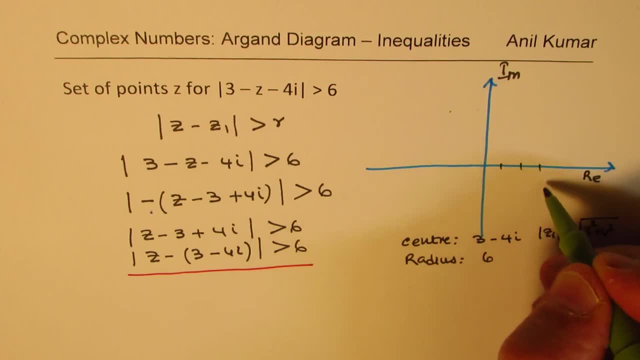 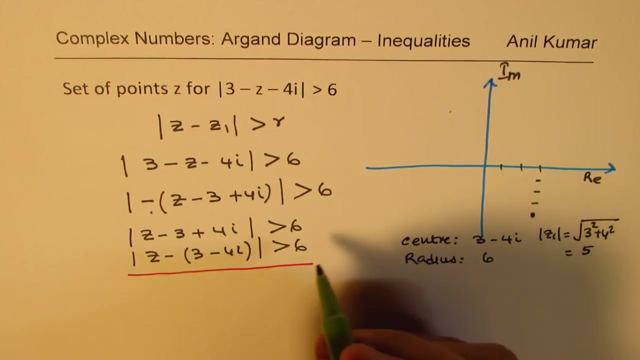 That means you go 3 units- 1, 2, 3, and minus means go down 1, 2, 3, 4, So that becomes your center of the circle. now, with this Center you Have to take radius of greater than 6 means this. greater than 6 means we are not including the circle. 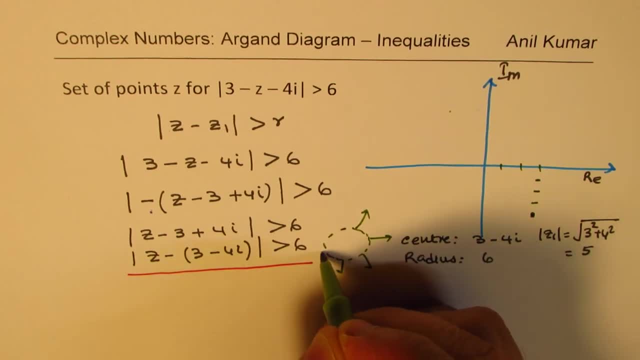 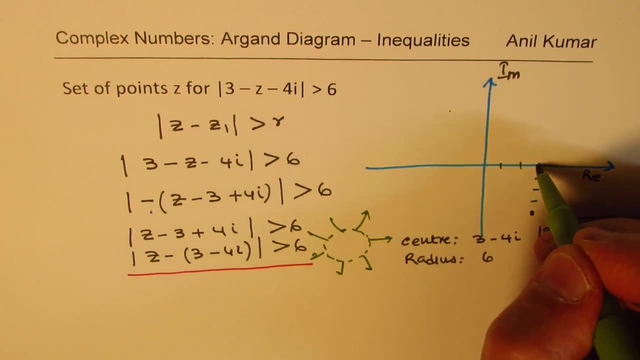 But we are saying everything outside. This is what our Inequality is indicating. so so we have to make a bigger circle. So let's just Make this 4 and 2 more units. that should be good, Correct. So this is from here, 5 units. So it is kind of going to cut across like this, correct? 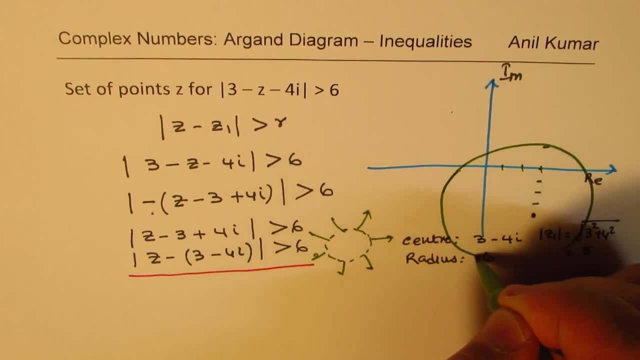 Okay, Okay. So I mean I'm just making one. So I mean I'm just making one. I know it's not perfect, but kind of gives you an idea, right. so What we're trying to say here Is that this, This is six okay, and the Center here is three minus four. i 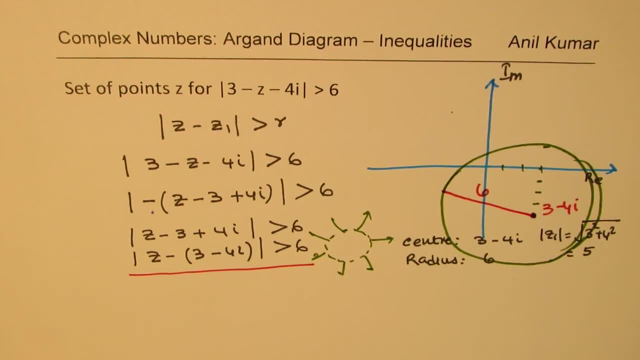 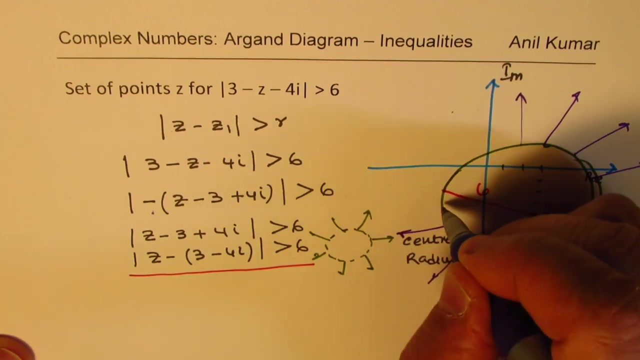 and The inequality. how should you sketch it? you have to sheet outside So it is greater than so. that is the inequality which we are talking about, right? nothing inside, not even including the periphery, correct? so that is how you are going to sketch. make it dotted if you want to.